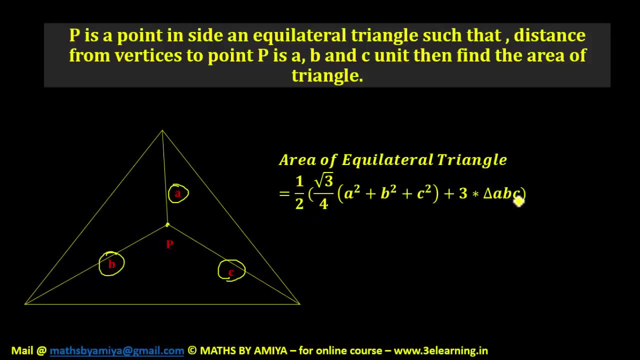 area, other side a, b, c for two. if sides are a b, c, these are triangles area. if the sides are a b, c, this is quite easy to remember. how comes we have half and root three by four is nothing but equator triangles area. root three by four: a, square b, square c, square a, b, c. say equator triangle by now. 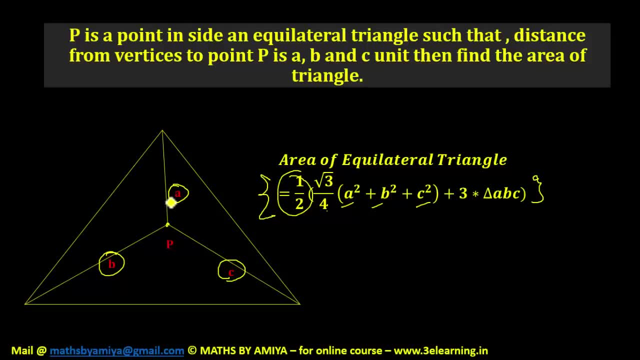 area nikaalo sabko add karo, and ABC se ek triangle banao. usse area nikaalo sabko add karo, and 2 se divide kar do. yahi hamara formula hai and isse use karta hai. iss question ke. 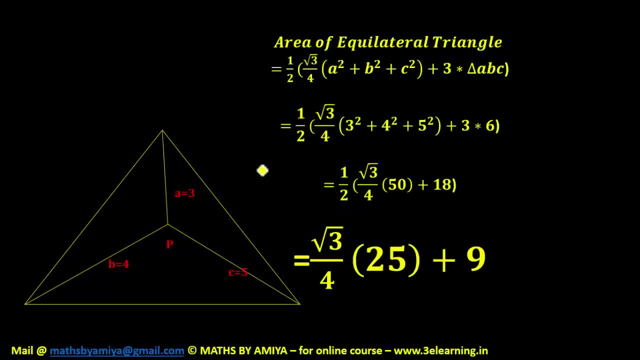 liye, and if you know the formula you can solve within seconds. So here the question is: ABC are nothing but 3, 4, 5, mai formula mein put karta hu: 1 by 2 root, 3 by 4, 3 square plus 4, square plus 5, square plus 3 into 6, how we get the area? 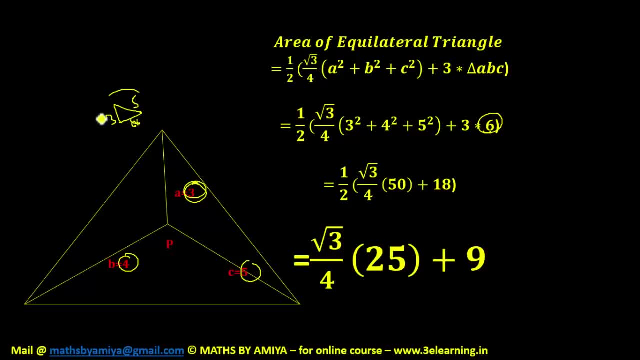 is 6, since this is nothing but the sides of a right angle triangle. so area is half into 3, into 4, so the 6, if sides are not the right angle triangle, use the heroine's formula and get the area, solve the values and get the answer hardly. 10 se 15. second lagenge. 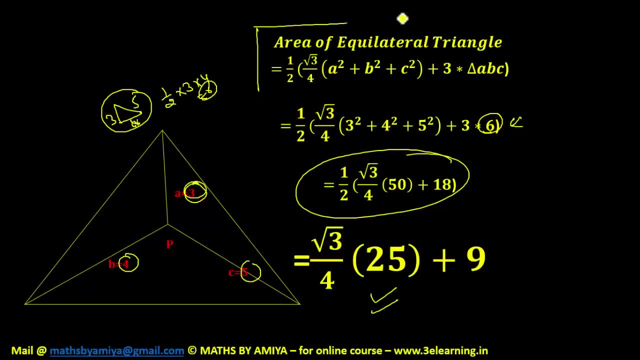 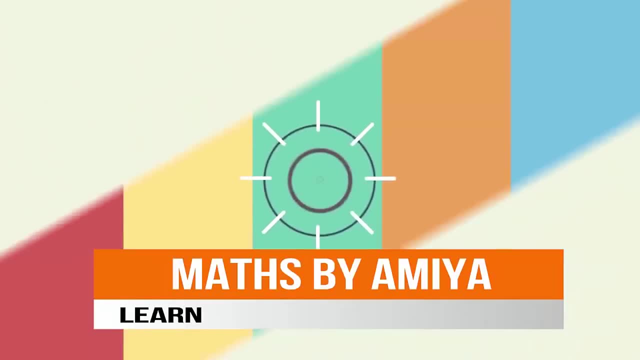 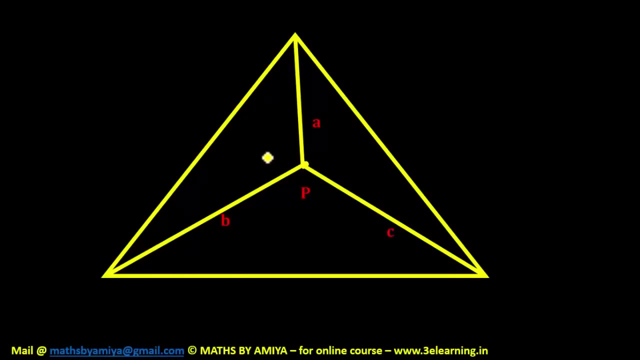 it would take hardly 15 seconds. So please note down this formula for examination. now it's time to understand the concept. First of all, we do some constructions assume triangle's vertices are ABC and the area of this one is X, area of this triangle is Y, area of this triangle is Z. so we need to 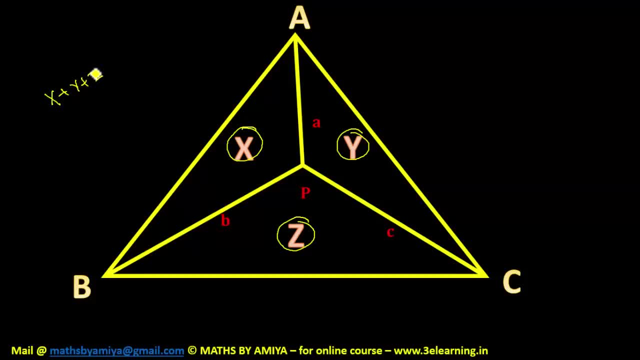 find the value of X plus Y plus Z. so our aim is to find the values of XYZ. okay, Now we will do some construction. if we have PBC, hamare pass ek triangle hai maine PBC ka rotation diya. and P point ko yahan dalaa C yahan rakhaa. B point ko yahan pe dal diya. 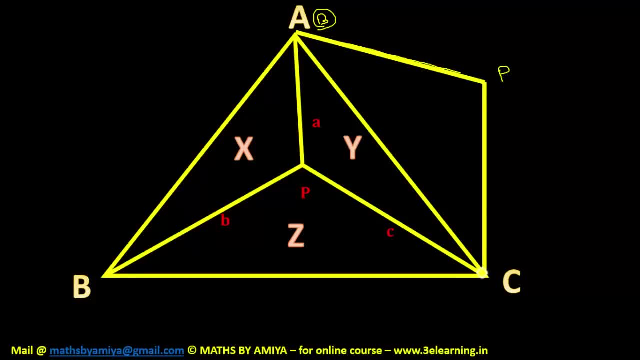 so this one is nothing but PB, this one is nothing but the PC and ye aapka BC hai. and BC is equal to AC because it's an equilateral triangle, so wo complete overlap karega. so can I say: if this angle is theta to ye angle, b theta hoga. why comes? because it's PCB. and 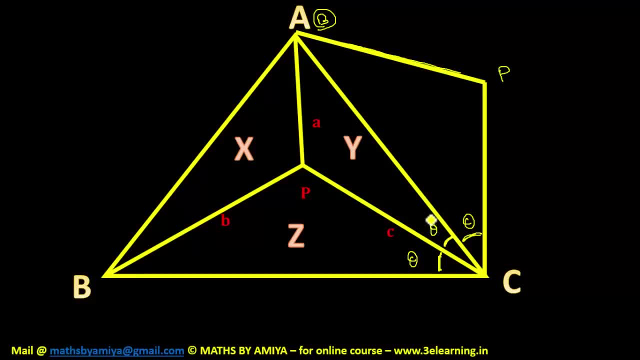 we do not know this angle, but we can see. if this angle is theta dash to theta dash, theta plus theta dash is 60 degree. we can say theta plus theta dash is 60 degree. so if we join p to p point- that is a rotation- say the p dash. so p to p dash is nothing but. 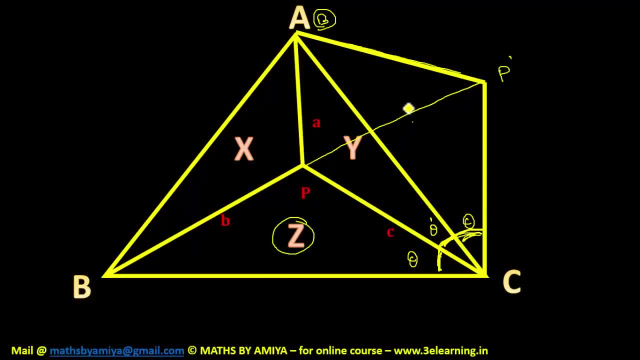 equilateral triangle and the pbc area is z to ish triangle ka bhi area z hoga to. we can say: y plus z area is nothing but the area of equilateral triangle whose side is c. how comes equilateral triangle? because isosceles triangle one angle, 60 degree. so the area of 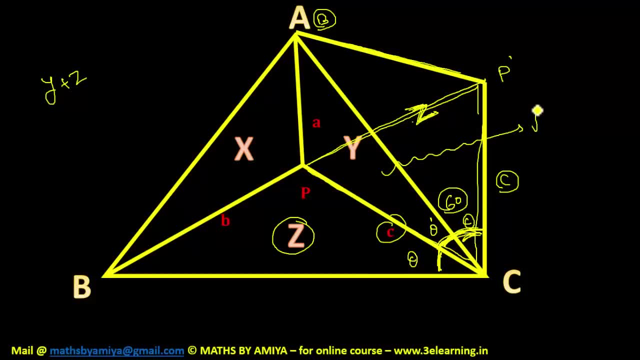 this region that is, pc p dash is root 3 by 4 cs square and if this one is equilateral triangle, p to p dash is nothing but c. ap is given a, pb from here is b, so we can find the area of ap p dash. this triangle is the area of triangle with the side abc, so we can say: 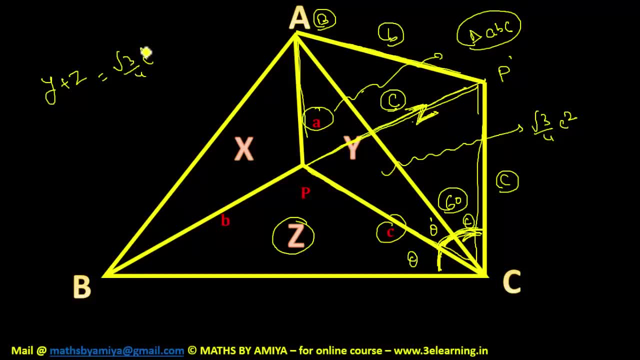 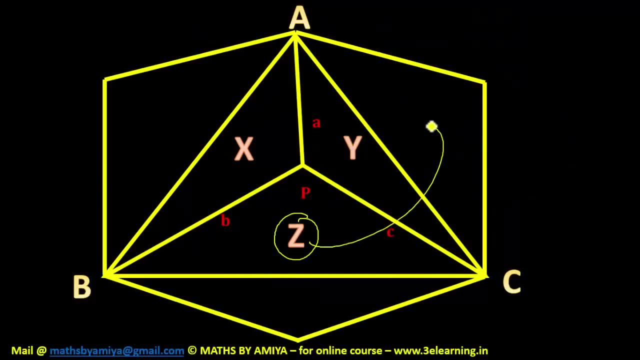 y plus z is nothing but root 3 by 4 c square plus area of triangle abc. with the similar construction we can find yz main. yaha pe y construct karunga. yaha pe x construct karunga. we can find all the area. so this one is my figure: agar maine z ko yaha construct kiya. 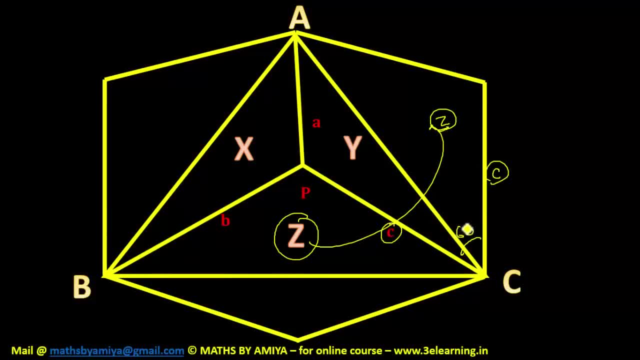 tha with the rotation of c c 60 degree. my area was root 3 by 4 c square and the upper area was nothing but the triangles area. abc and the area of triangle is nothing but the same and this one was the y plus z. agar aap y ko yaha construct karte ho with the side. 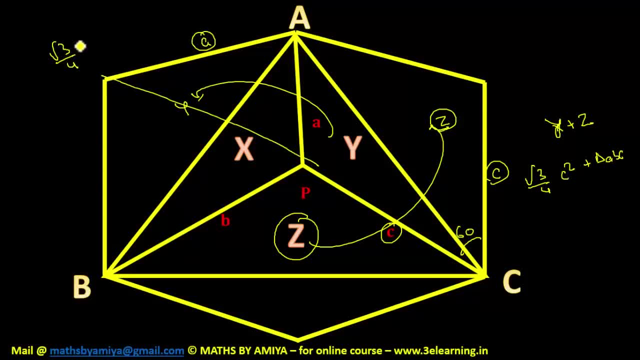 aa common. so we can say: this one is the root 3 upon 4 a square plus again we have nothing but a, b, c triangles area. and this one is what y yaha pe aaya hai to x plus y ho jayega agar aap x ko yaha construct karte ho to. we can say: x plus z is nothing but b ko maine yaha. 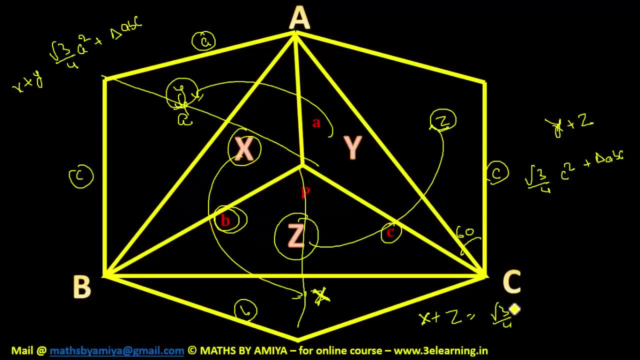 construct kiya equilateral triangle banaya hai. root 3 by 4 b square plus. this one is b, yaha, c, yaha, aapka a hoga, because x utke yaha pe a gaya hai. so that is triangle abc. agar aap teeno ko add keroge to, we can say twice of x plus.